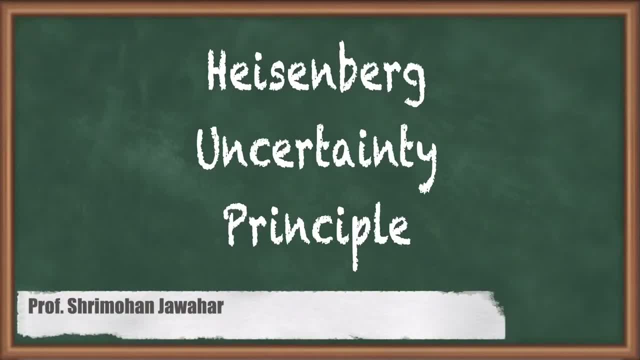 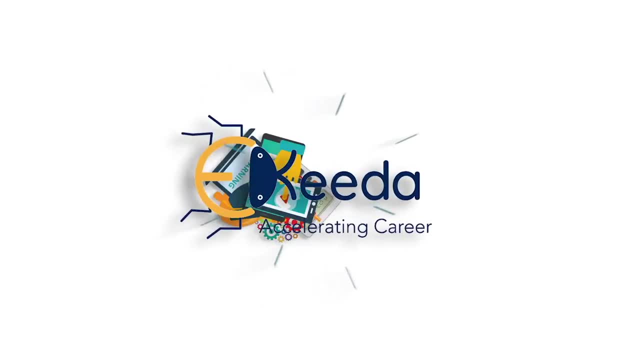 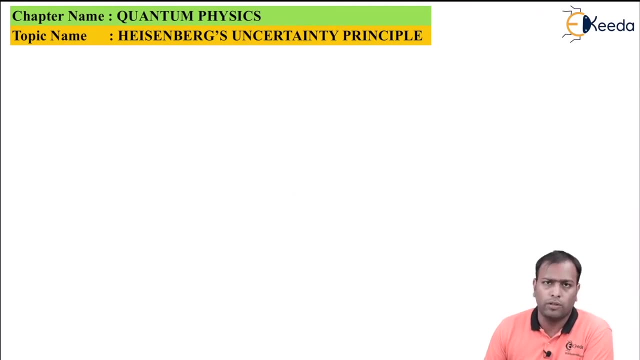 Hello friends, in previous classes we studied about the de Broglie's hypothesis, and in earlier classes we also studied about the atomic structures: Thomson model, Dalton's model, Rutherford's model, finally the Bohr's model. but unfortunately none of them were able to predict the actual position of the electron. Well, this was, however, been ruled. 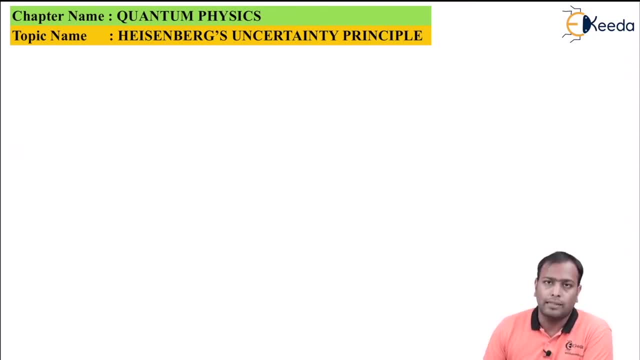 out by a German scientist, Heisenberg. He said that electron can never be found at a particular location. So in today's class we'll be just exploring them in detail. So stay tuned. Heisenberg's uncertainty principle: The principle states that it is not possible to know. 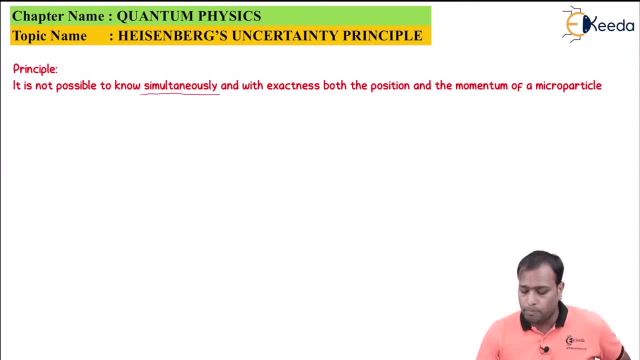 simultaneously the exactness, both the position and the momentum- of a micro particle. Now, well, to make this simple, we need to know the exact position and the momentum of a micro particle. Now, well, to make this clear, let's take an example of a ball. I have a ball which is at a location here. Let's say the. 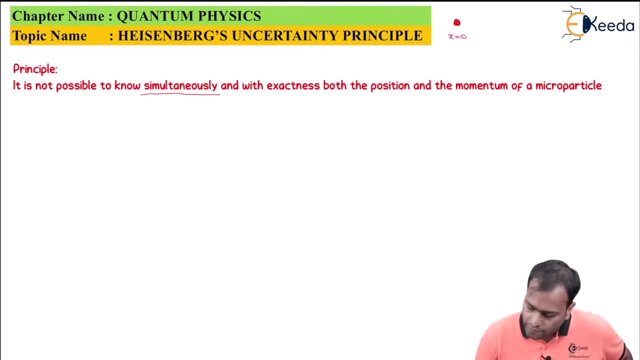 location x is equals to zero and I have already told you that it moves at a speed of five meter per second. Assuming the mass of the ball to be one kg, you already know the momentum. The momentum is five units. Now if I tell you to find out the position of the ball after two seconds, 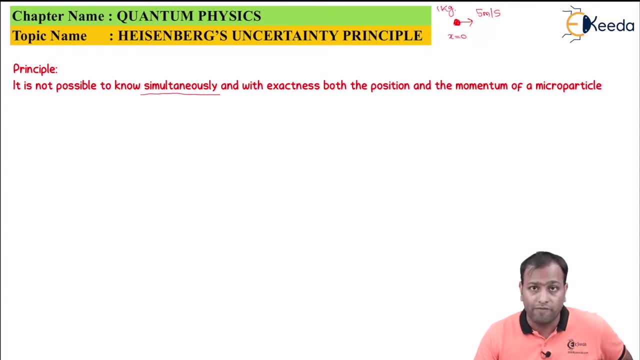 it won't be that difficult, because you know that if it is moving at five meter per second, of course, after two seconds it would be at the distance of 10 meter from the starting position in here where your ball is located. Well, it looks quite simple. Now, why is this possible? 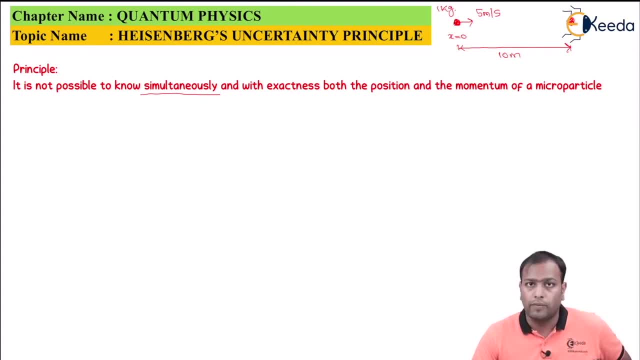 This is possible because we are dealing with real world objects. For real world objects, the objects stands there and there. They don't deviate from their position. Well, how to understand this? as an example, Well, if I ask you to find out the position of the ball, 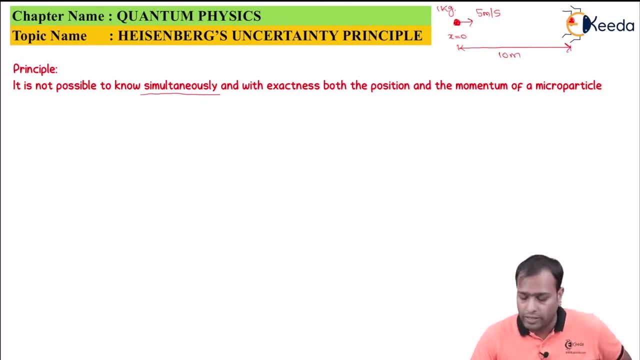 it was quite easy. But what if the ball was already shaky from its position? Well then, you could never say that it would reach just at a distance of 10 meters from its starting position. It would be somewhere up or down. Well, the only difference between real world objects and 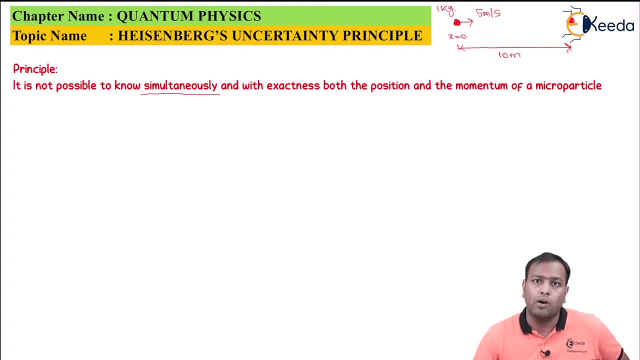 atomic objects is: atomic objects have a wave nature. We already have studied that the wave nature for real world objects is not that significant, But for subatomic particles it's very significant. So basically, what we mean to say here, we mean to say here is: 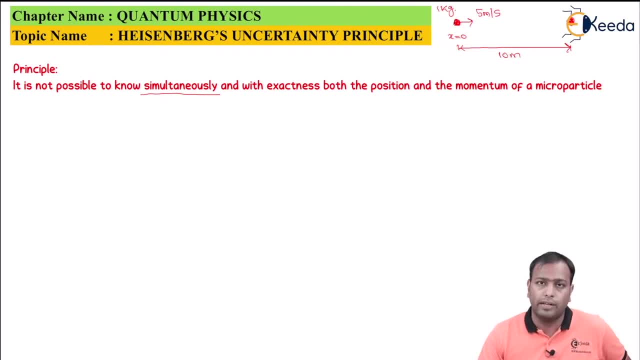 okay, if you know the exact position of the ball, then definitely you don't need to worry about what its future prediction would be. But if you don't know the exact position of the particle at time zero, you would never be able to tell what its future prediction would be. Now you know the 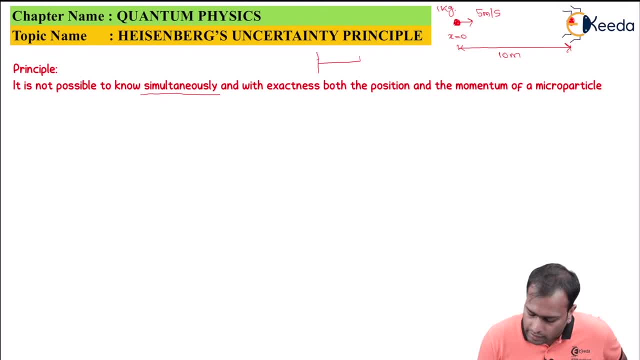 future prediction. Well, basically, a wave packet is nothing but as a cluster of waves combined together. Now this cluster of waves is nothing but as the probable position of the particle. Now here you already know that the particle is not known or there is always a uncertainty in. 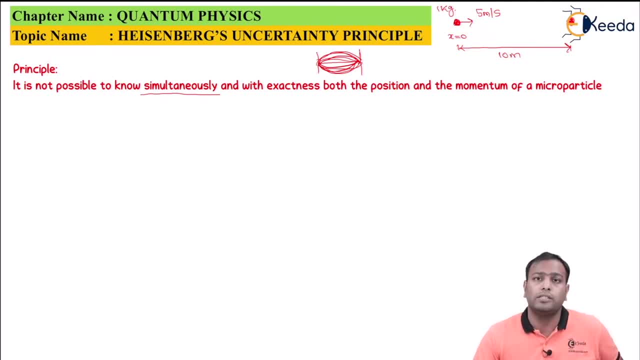 its position. Therefore, there is always uncertainty in its future prediction. Of course, if there is uncertainty in this future prediction, you cannot predict about the velocity. Well, Heisenberg was the scientist to first discover this and thus state this law, and thereby stating that it is. 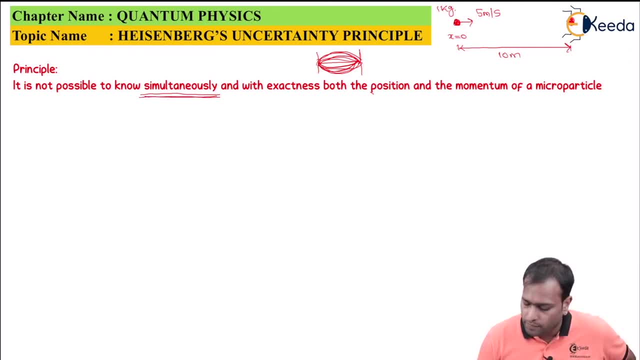 impossible to simultaneously know the position and the momentum. Well, if you try to accurately find out the position, of course you would not be able to find out the momentum, Whereas if you want to find out the exact momentum, you would be losing your position on position. 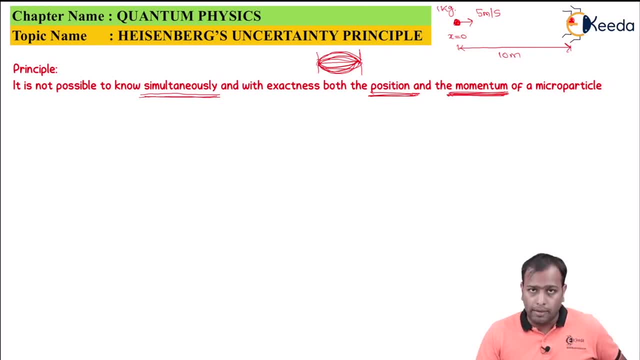 So basically, finding both the things simultaneously for subatomic particles is impossible, And the mathematical statement to this is: delta x times delta p is greater than equal to h upon four pi, where h is a Planck's constant, Delta x is uncertainty in distance, or you can say in position, It is related to position, and delta p is uncertainty with respect. 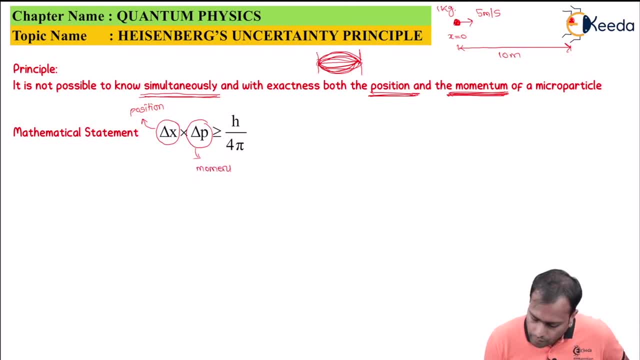 to momentum. So the law by Heisenberg states that the difference in the distance or the position, or the uncertainty in the position times, uncertainty in the momentum, is always greater than equal to h upon four pi. Now, well, this is how the graphical representation looks like. As you can see, as I am, 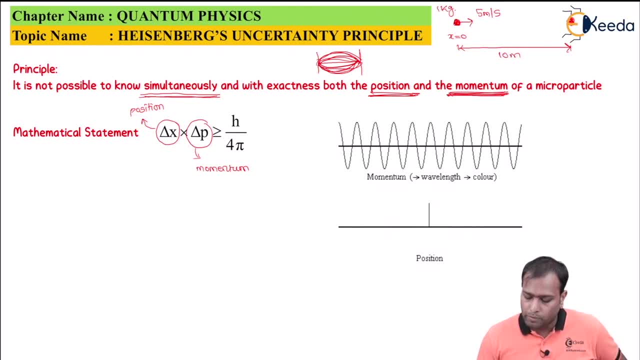 trying to accurately determine the position, my momentum widens, whereas if I am trying to accurately determine the momentum, my position widens. This trade-off is always constant. Now we know that momentum is nothing but as mass into velocity. p is equals to m times v. However, mass of the objects 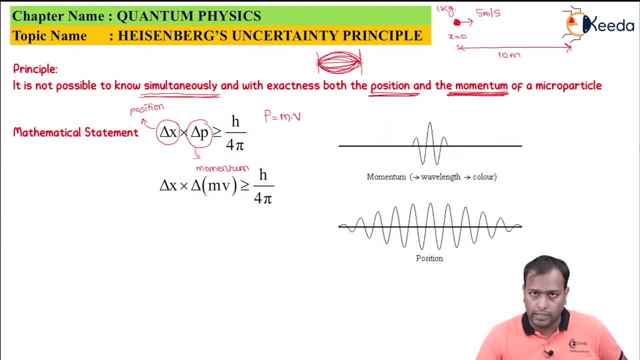 does not change significantly, but velocity does change. So I would say that delta x times delta times of m v greater than equal to h upon four pi. Now taking mass constant or outside, this would be my equation: delta x times delta v greater than equal to h upon four pi m. Now let's take two cases. 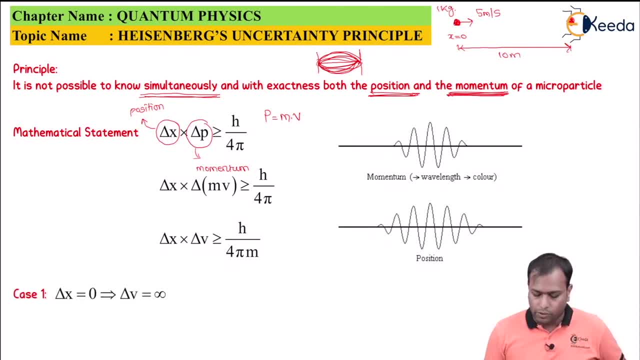 for instance case one, my delta x is equal to zero or there is no uncertainty in the position, which means I am able to determine the exact position of the particle. So in that case my delta v would go just to maintain the constant equation. So if my delta v is infinity, of course there is again an 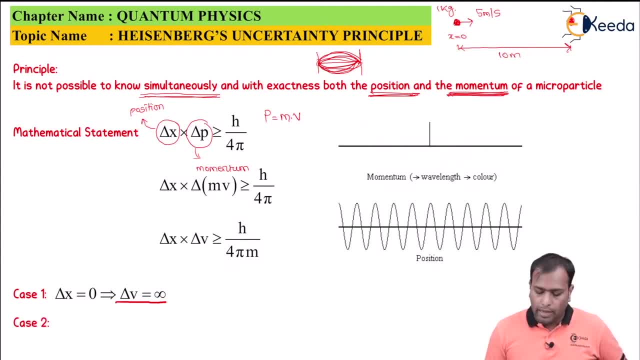 uncertainty In case two, when I am able to determine the exact velocity. so there is no difference in the velocity or there is no deviation in the velocity, of course my delta x would go equal to zero. So basically we mean to say that there is always a trade-off between 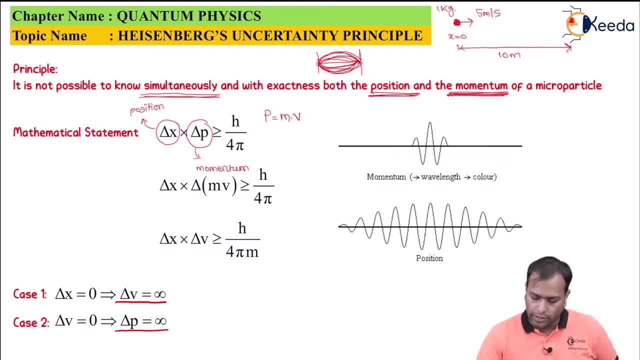 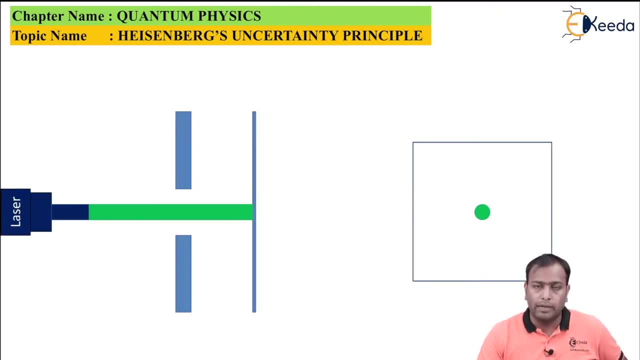 the momentum and the velocity. There's a trade-off between the position and the momentum. Let's understand this by a simple experiment. that was a single slit experiment. Now this is an experimental setup for Heisenberg's uncertainty principle. Here you have the two slits. here is 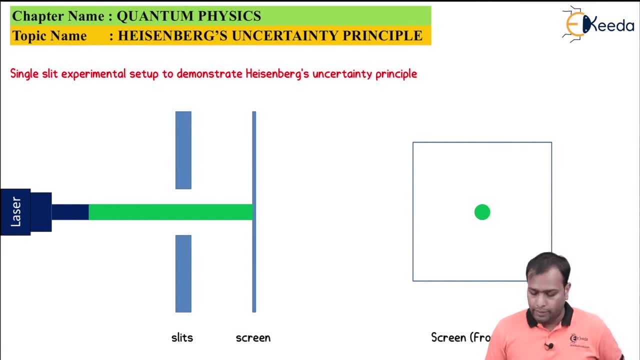 the screen, and this is the front view of the screen. Now, what we will be doing is we would be narrowing down the slits so that my beam gets narrower and narrower, and I would be significantly watching the difference between the initial image and the final image on the front view of the 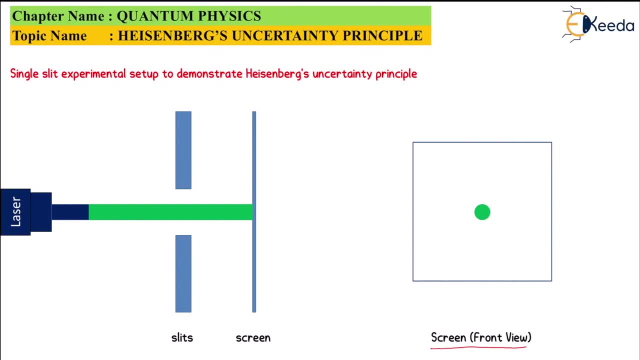 screen Now as my slits go further. as you can see, there's no change as of now, because I am still wide enough for the beam. Now, as soon as I touch the beam here, you can see what is happening. I'm actually- this is my delta x. I'm actually trying to minimize the uncertainty. 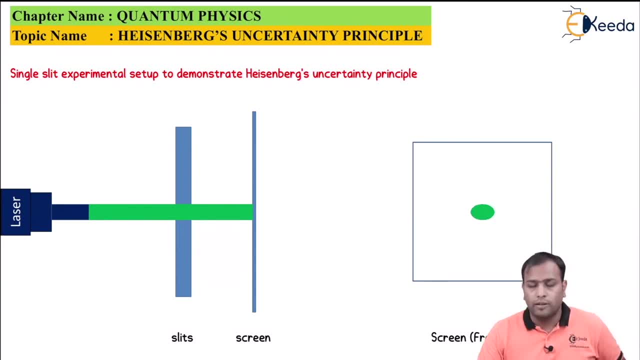 in the position. So what happens? the image widens as it goes further. the image widens further. So if I'm trying to accurate the uncertainty in position, my momentum changes and hence this image wider. In the opposite way, if I widen the beam, what happens is the node gets 80.. Retake for. 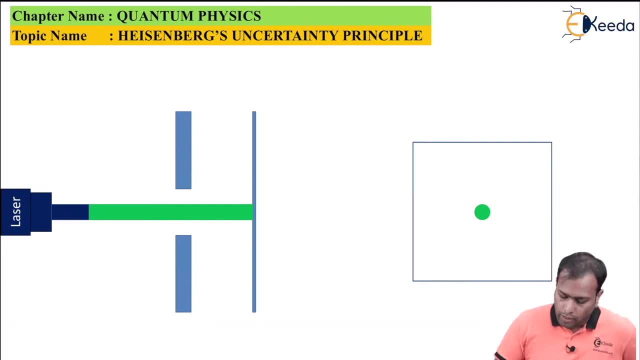 single slit experiment by Heisenberg. Now, this is an experimental setup for single slit to demonstrate Heisenberg's uncertainty principle. Well, to understand the Heisenberg's uncertainty principle, real world objects are of course not the case, because there, we already saw, there is a 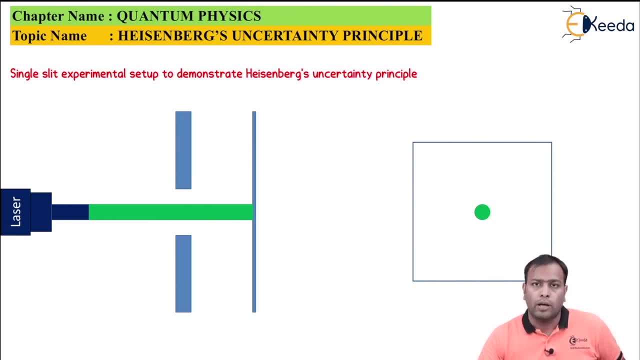 de Broglie wave and the size of the object Now, but to determine the uncertainty principle we'll be using light. This is an experimental setup of a single slit wherein a laser beam is projected on a screen which passes between slits. Now we would be narrowing down the slits. 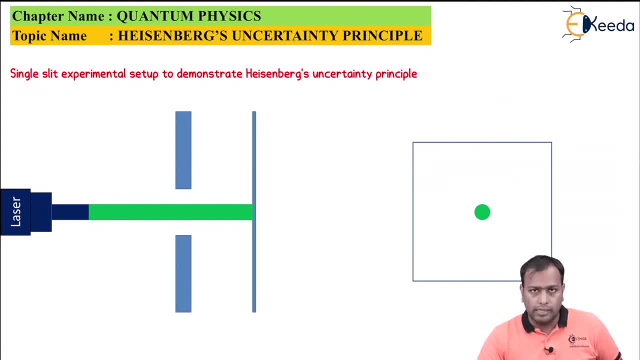 further to minimize the uncertainty in the position. Now, as we know, delta x times delta v is always greater than or equal to h upon 4 pi m. So now, as my delta x goes down, my delta v goes up, just to maintain the Heisenberg's uncertainty law. So what happens when delta v goes?